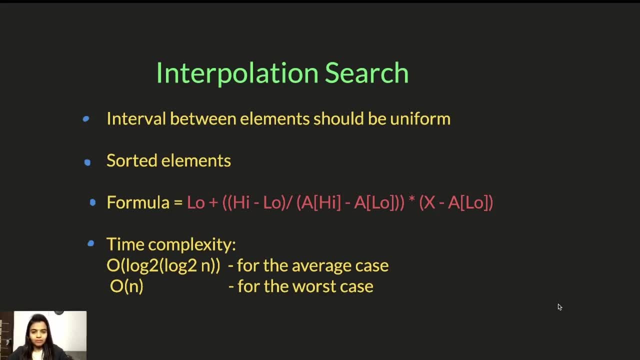 description. So there are a few things that you have to keep in mind for interpolation. search, That is, the elements of the array should be uniformly distributed. So in other words, the interval between each element in the array should be uniform. Okay, like. 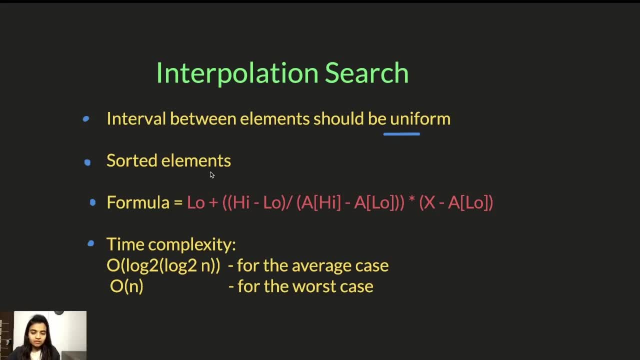 in same like binary search. even for interpolation search all the elements have to be in sorted order. Now, in binary search what we used to do is find the left element, the right element, divide it, add them and divide by two and find the middle element, right. So 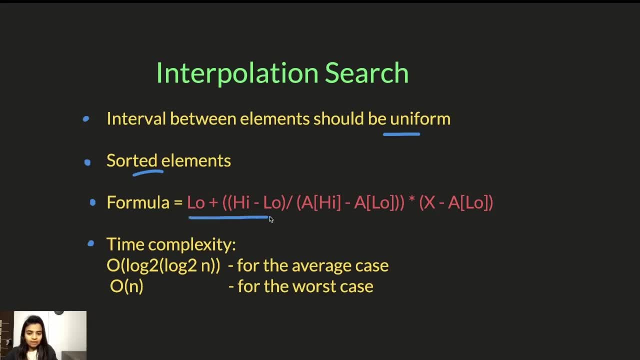 binary search is very similar to interpolation search, So in this video I'll be talking about. So binary search is very similar to interpolation search, So in this video I'll be talking about. but here we have a formula. What this formula does is it tries to give you an index which 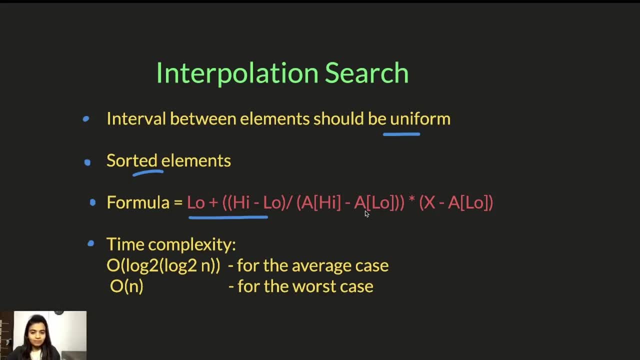 is very close to the key. I will explain it further with an example. So time complexity is O of log 2 of log 2 n. This is for average case and for worst case it is O of n. Now I'll explain interpolation search with the help of an example. 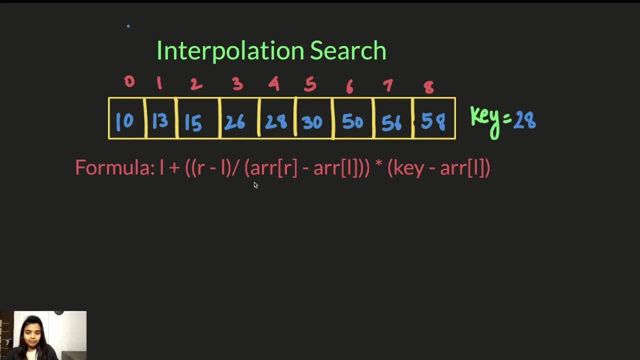 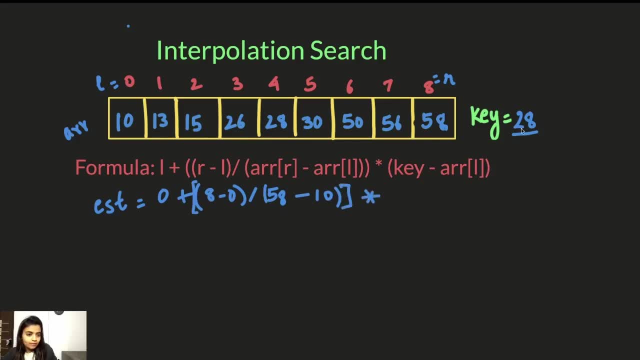 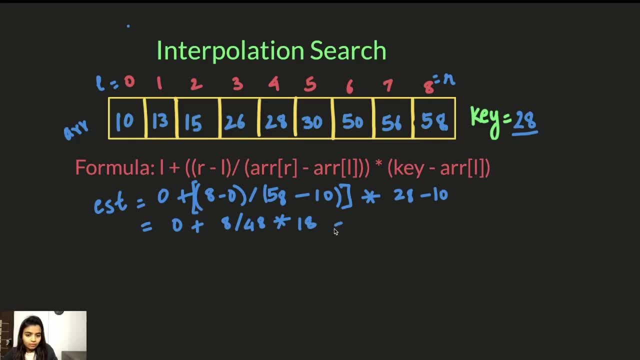 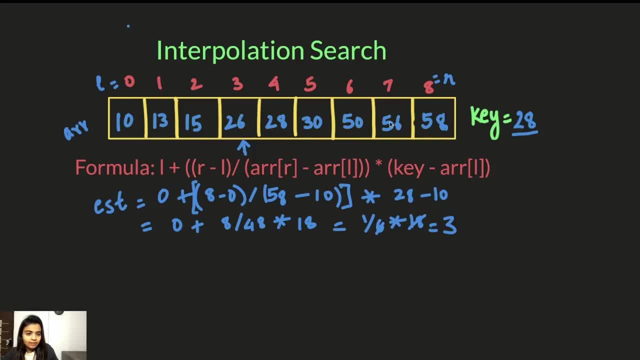